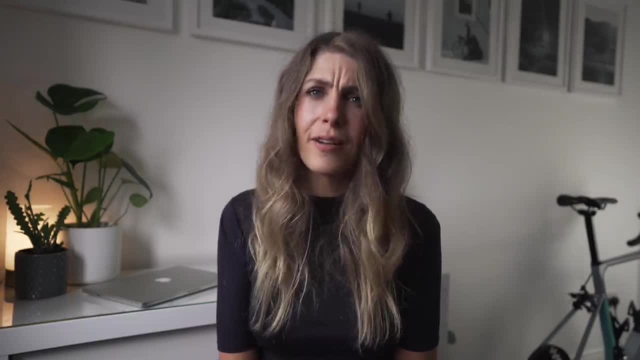 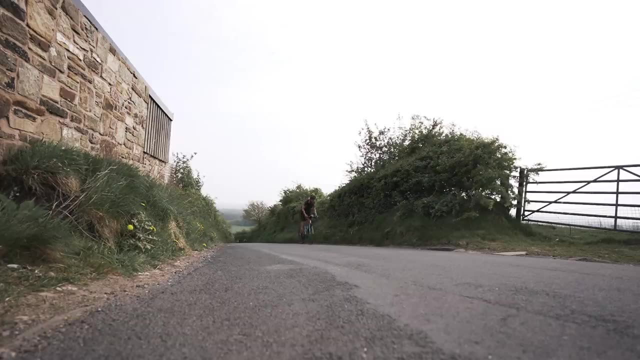 standing on a climb. it just felt really bizarre to me and it just felt really unnatural. So I would say from the very start, just get used to climbing out of the saddle, because as you kind of progress, you will want to climb out of the saddle for a number of reasons. So one, if you get on a climb, you're going to want to climb out of the saddle for a number of reasons. So one: if you get on a climb, you're going to want to climb out of the saddle for a number of reasons. So one: 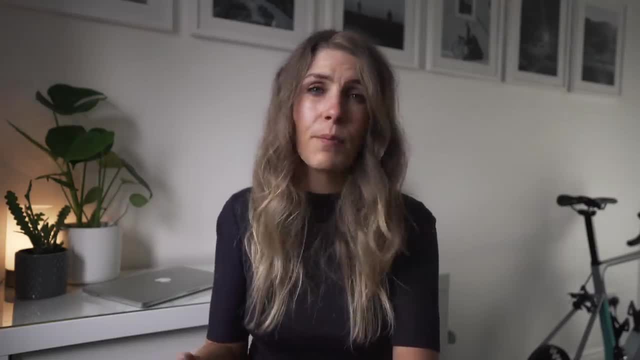 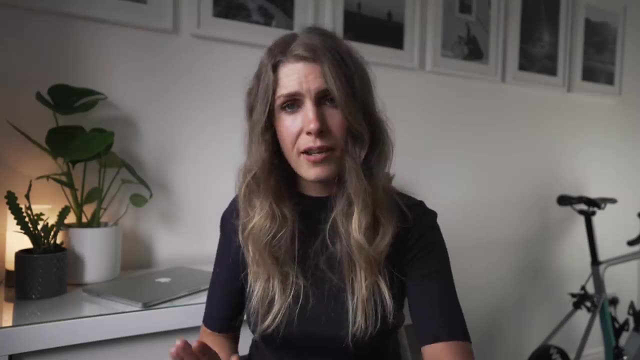 if you get on a steeper climb it's just easier just to kind of move the bike and get up that climb. You're also able to put more power down because you stood up and you're able to kind of put more power through the pedals And also it just relieves pressure from your saddle. So if 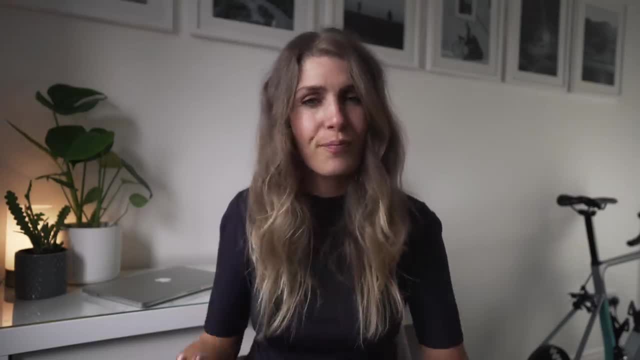 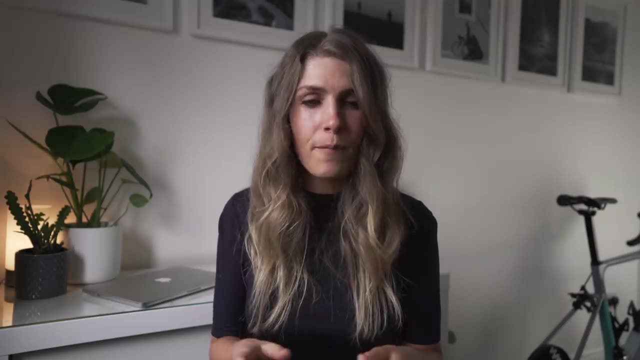 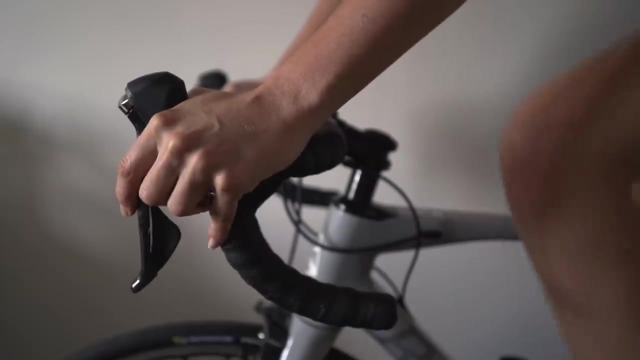 you've been climbing for a long time. you just want to get out of the saddle and just kind of relieve that pressure. Know your gears. You want to know which way your shifters work to get in the right gear for climbing. And I know that when I first started I actually had no idea like what. 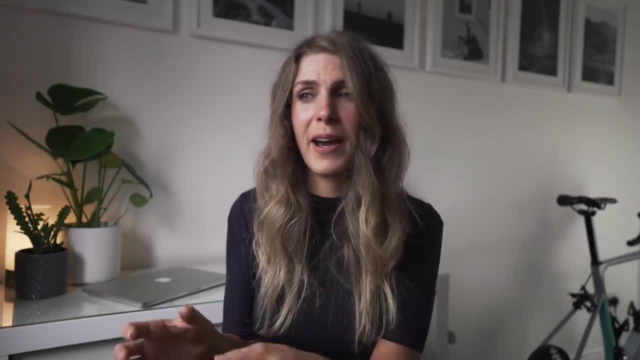 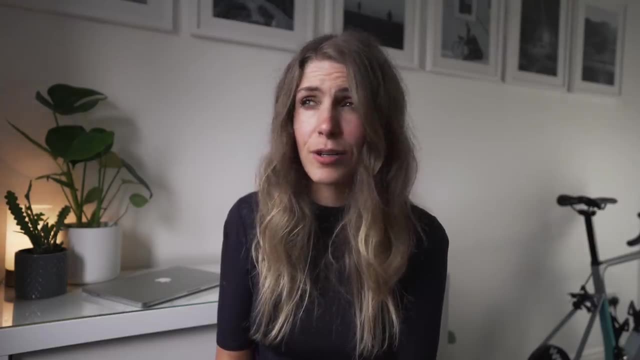 the gears meant on the bike. I remember when I actually bought my first road bike I asked the guy in the shop and was just like so how do the gears work? And this guy looked at me, just gone out like you'll figure it out. But I'm going to help you because I wish he just told me and helped. 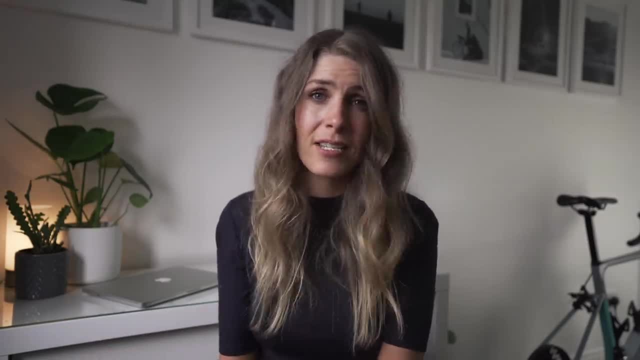 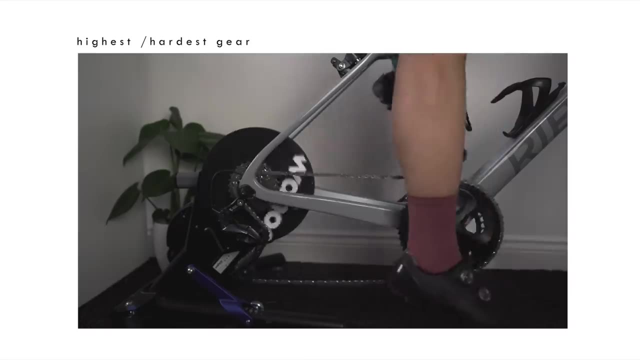 me understand. It might seem obvious to some people. It did not seem obvious to me of like, which was the gear that I use on the climb? which was the gear that I use when it was flat, If you're at the big chainring at the front and 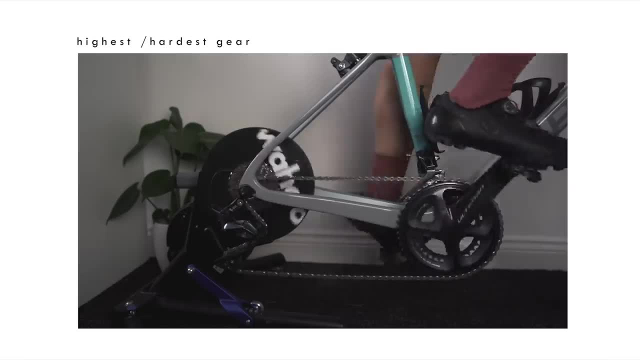 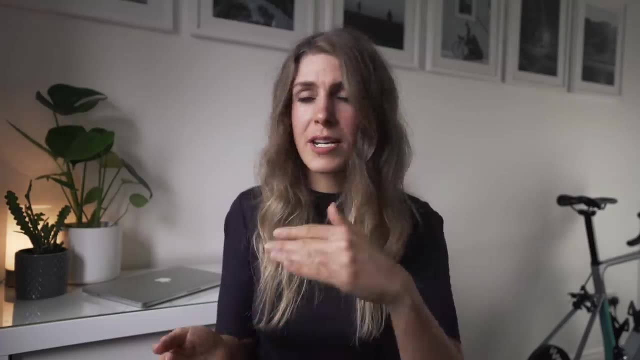 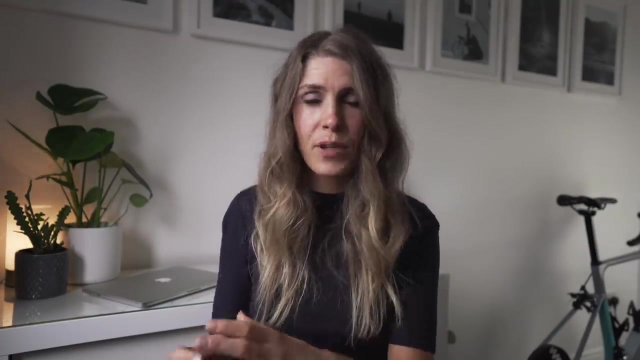 the smallest cog at the back and the cassette on the back wheel. that is your kind of hardest gear. So that means if you are on the flat or on a descent, that is the gear that you want to be in. If you are climbing and you want the lowest or the easiest gear, you want to be at the smallest. 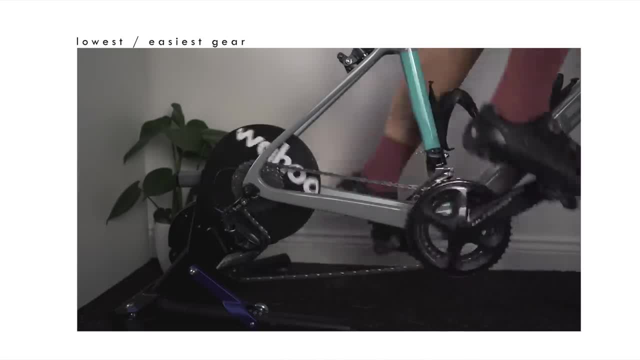 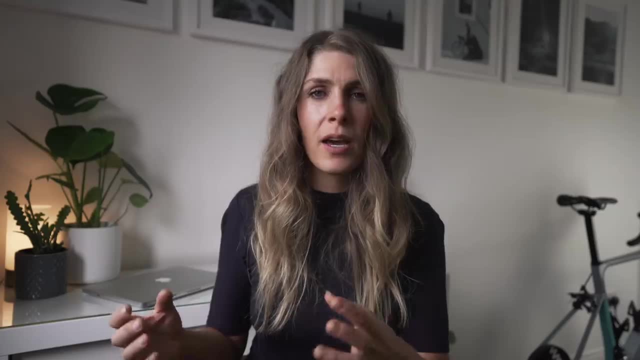 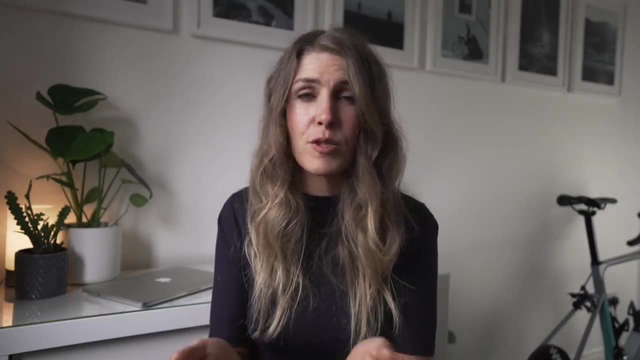 chainring at the front and the biggest cog at the back of the cassette And again, I guess, tied in with that, you can actually change these ratios So you can buy different size chainrings and different size cassettes to kind of get the perfect gear for you. So if you live somewhere flat, you don't necessarily going to need a big cassette, Whereas if you want to ride loads of hills, like I do, I have a big cassette because I want to be able to ride up hills all day and not get any kind of massive fatigue in my legs or any kind. I don't have to. 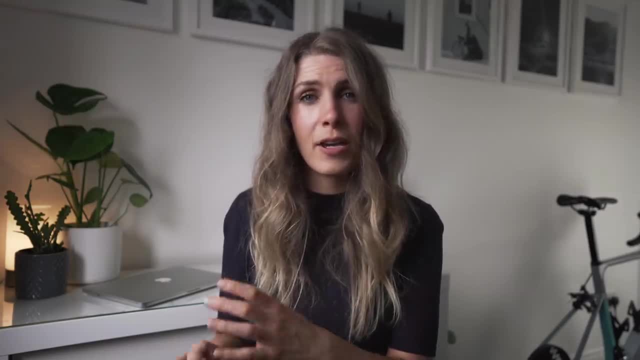 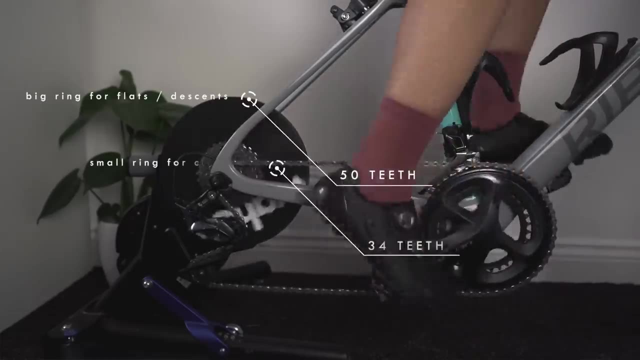 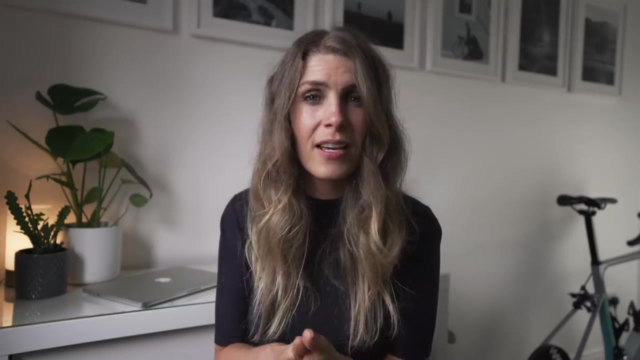 do that. So my personal setup for climbing is: I've got a compact crank at the front which is 50 teeth on the biggest chainring at the front and then 34 on the smallest, And then I have an 1140 cassette on the back which is actually a mountain bike cassette. Not many people do this, but yeah. 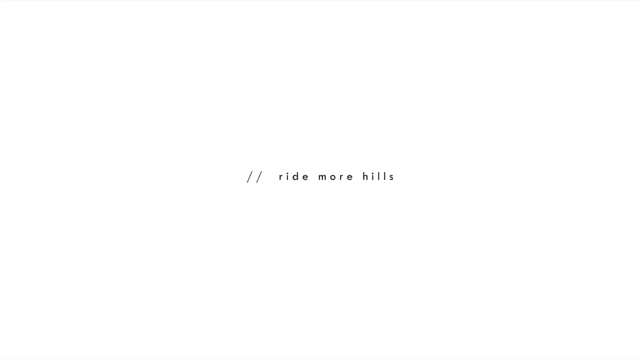 that's how I have it, because I like riding hills. The next thing is it's quite a simple tip and that is just to get out and ride them. Don't worry if it takes you forever. it's not going to be that easy, But if you're going to be able to do it, you're going to need a. 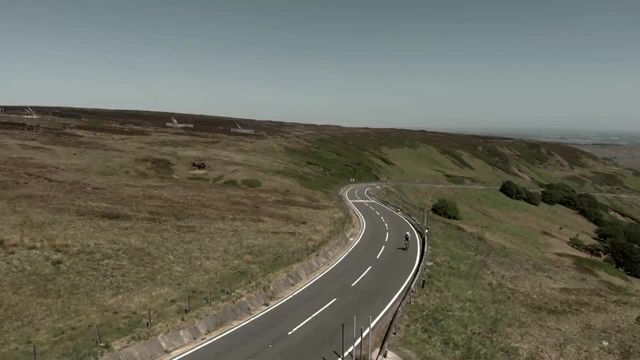 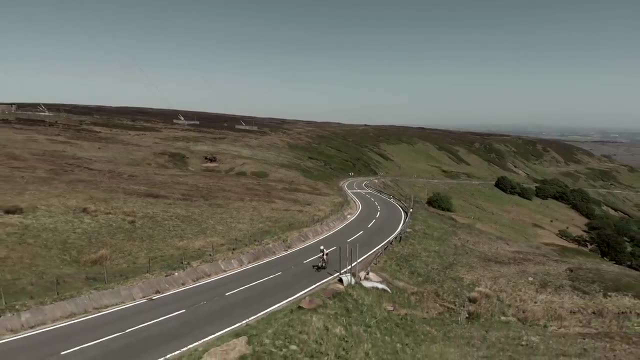 couple of hours to get up a climb. I've shared my story of how it took me two hours to get up like 5K climb. It doesn't matter. The fact is I was out there and I was doing it, And that's all you need. 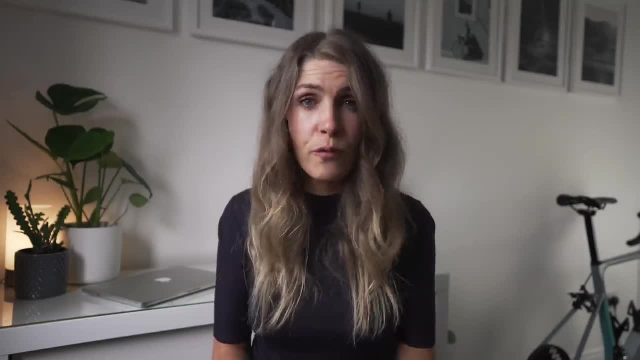 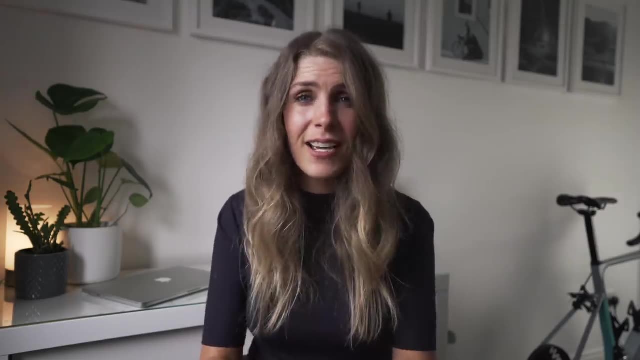 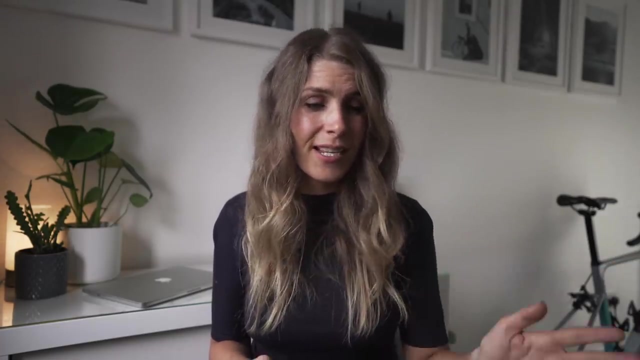 to do to get better is just practice them. The more you do it, the more comfortable you'll feel on those climbs and the faster that you will get. And I cannot cannot emphasize enough how important it was for me. I had one climb that was, and it's my favorite climb still. it's six kilometers And 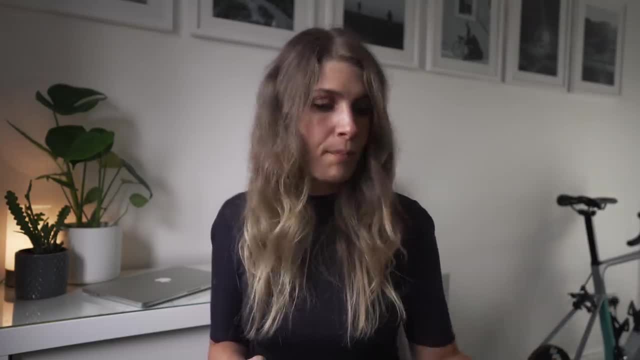 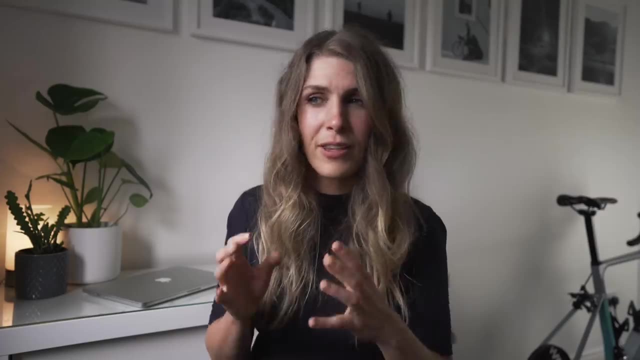 I just went back. I found that climb and I just kept going back and back and back because I wanted to get faster. And I did that for maybe three years when I first started cycling And having that kind of focus, just to keep going back to that climb. obviously I did others, but that one climb. 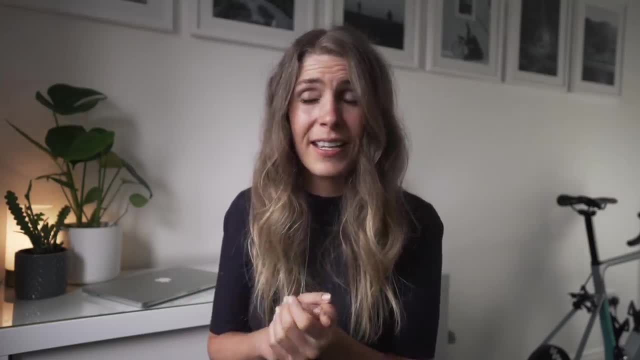 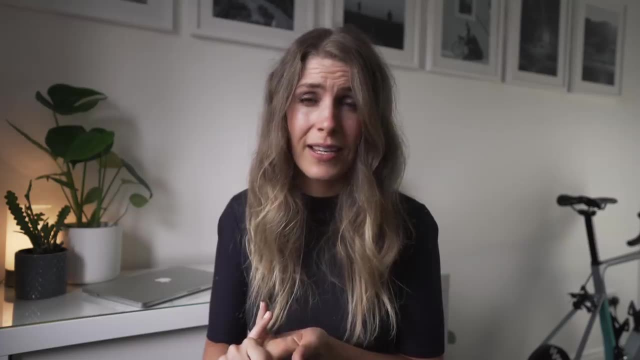 and my motivation to get a faster time on it. I just got so much fitter- Sorry, my finger cracked. then Got so much fitter, I lost- lost a lot of weight. I'm going to be doing cycling: weight loss. 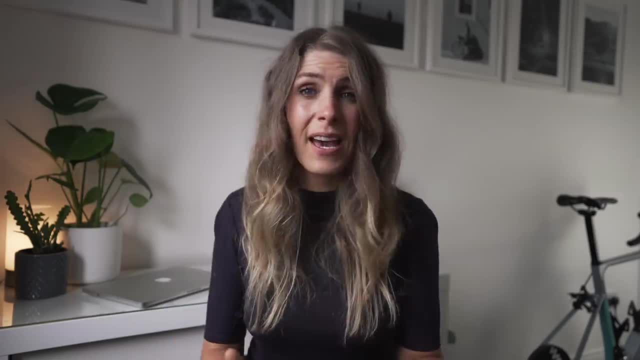 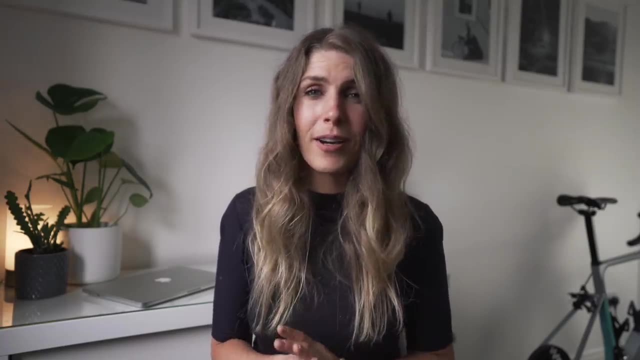 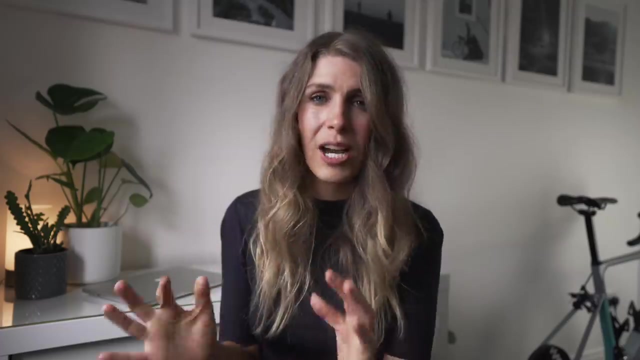 video as well, because I've lost about 35 kilos. But yeah, and most of that was down to just going back and smashing that, smashing that climb. So find a climb that you love and just keep going back, Because I promise you it does get easier. Also, I do have an ebook that's got a whole chapter. 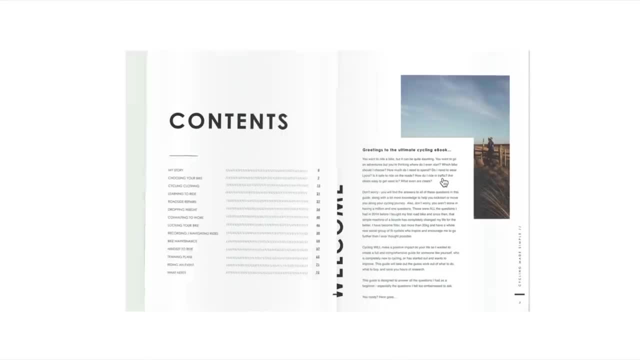 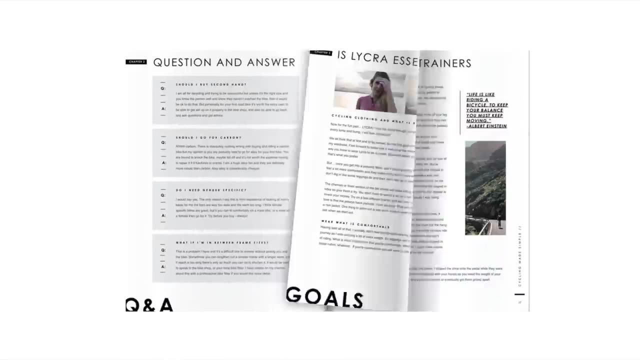 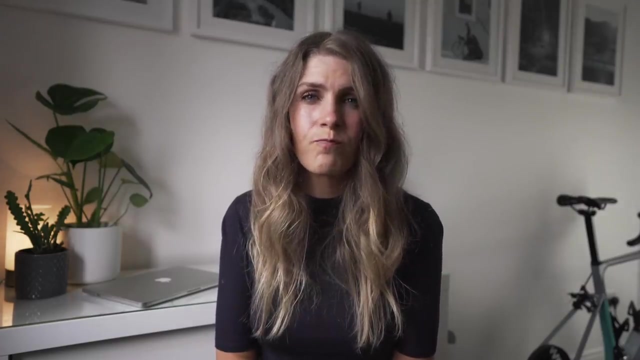 about climbing, And so, yeah, it's called Cycling Made Simple. There's a link to that in the description, but I'm going to be giving away one copy of that every single day over this 10 day period. All you need to do is just leave a comment in the comments and, yeah, I, you might win a copy.